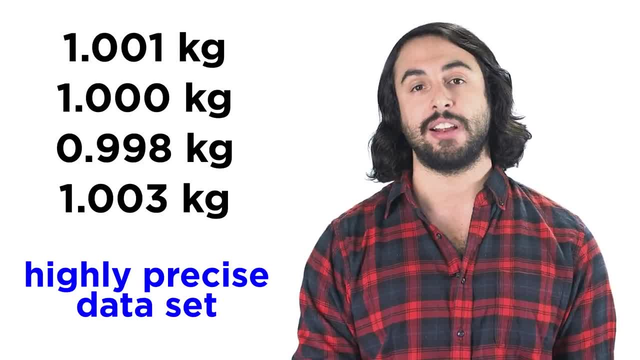 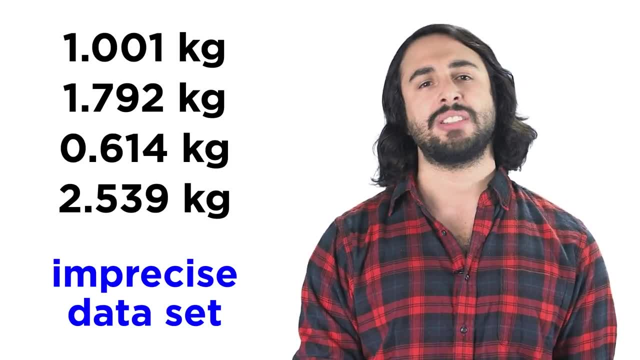 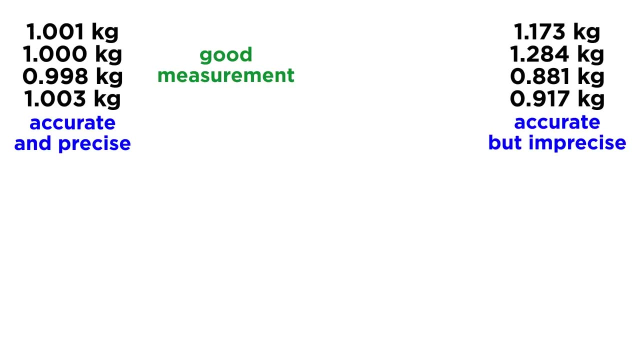 precise data set because all of the values are very close to one another. If there was much variance in the data, we would say it was imprecise. In this way, we can see that a data set can be both accurate and precise, which means good measurement, accurate and. 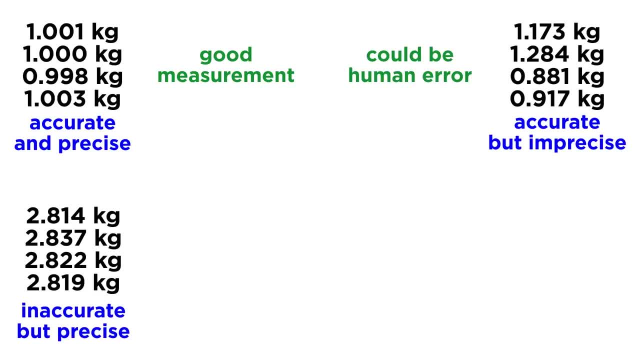 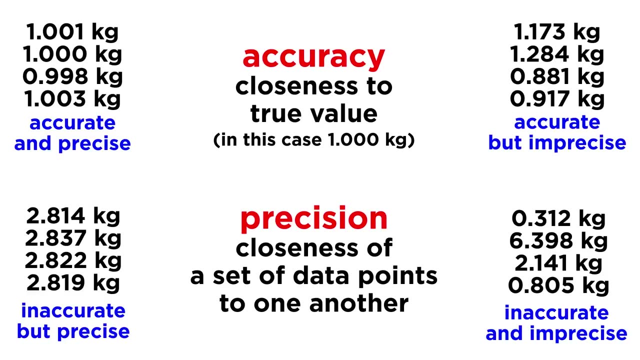 imprecise, which may simply be human error. inaccurate, but precise, perhaps due to faulty calibration of an instrument, or both inaccurate and imprecise, where everything goes wrong. Once again, these qualities depend on how close they are to the true value and 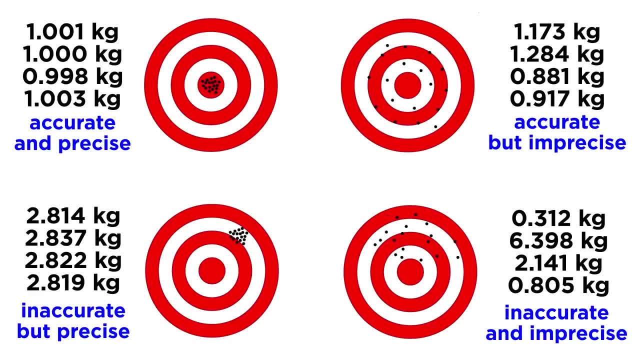 how close they are to each other. We can use target practice as an analogy. If we regard the bull's eye as the true value, we can see how the following results represent the different types of data sets we just discussed. Accuracy will mean that a data point is. 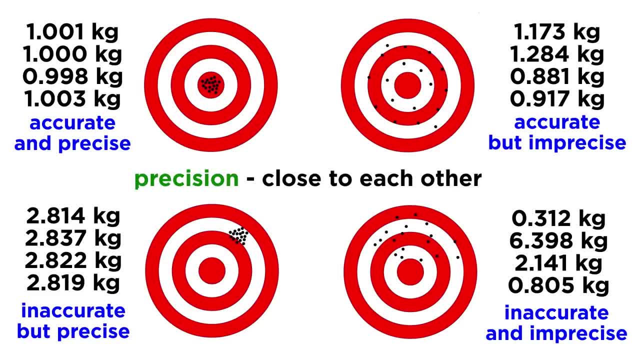 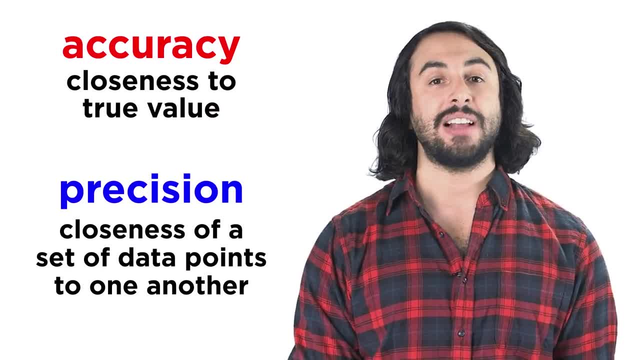 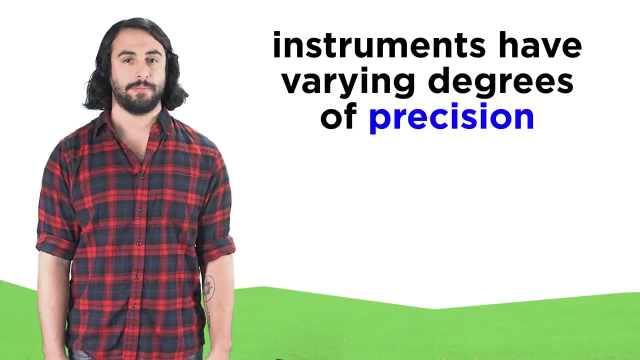 close to the bull's eye, and precision will mean that data points are close to each other. Now that we understand accuracy and precision in this context, let's learn about another context for the word precision. We could also talk about the precision of an instrument. 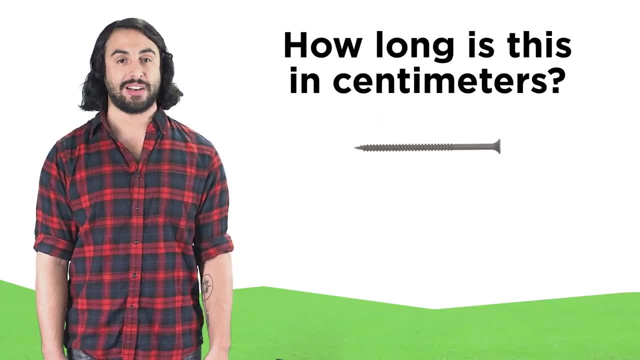 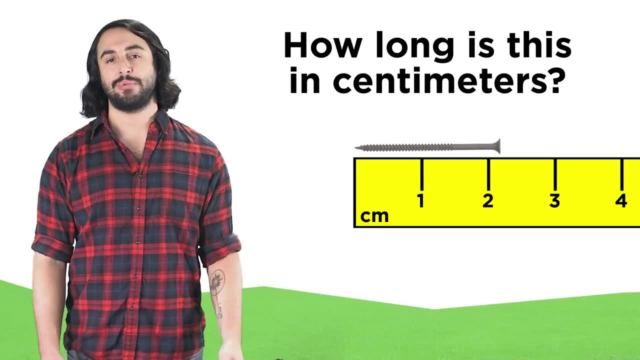 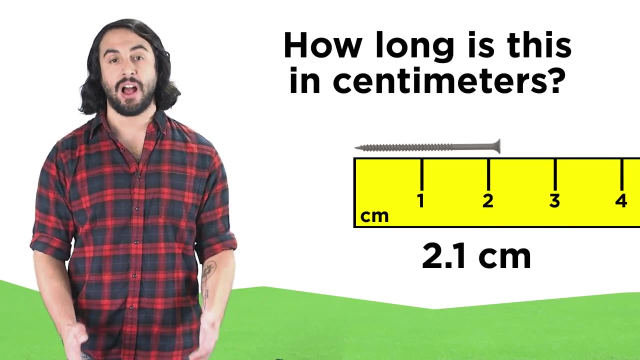 Let's say we want to measure the length of an object in centimeters. This ruler displays centimeters, so we could say that this object is between these two points, These two centimeter markings, and then we could estimate one more digit beyond that. 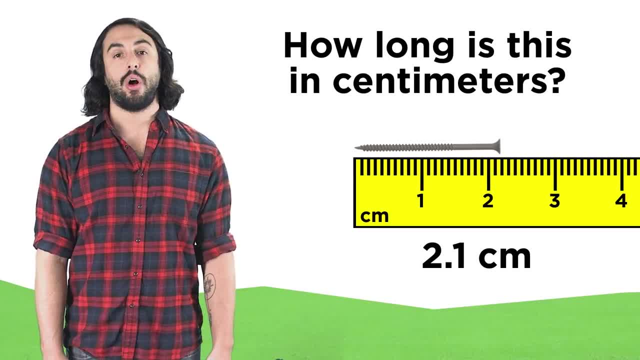 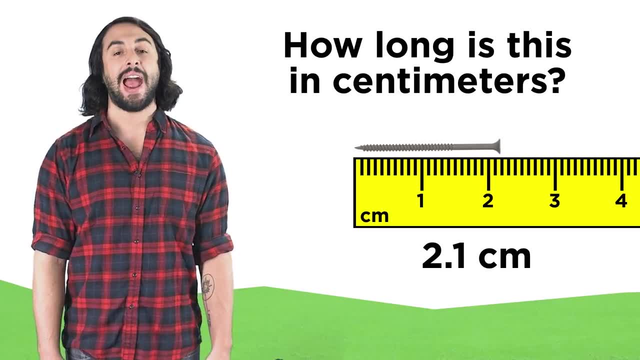 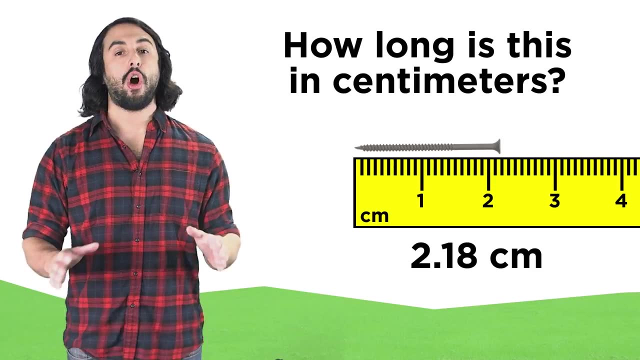 the tenths place. Let's say that the ruler also showed tenths of a centimeter. Then we could reliably report our value to the tenths place and now estimate the hundredths place. This is because when taking measurements, we always estimate one digit beyond the scale. 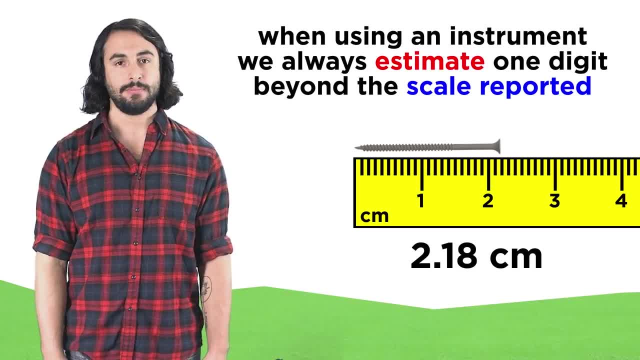 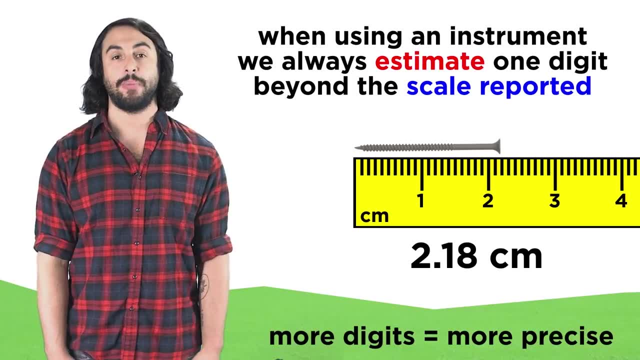 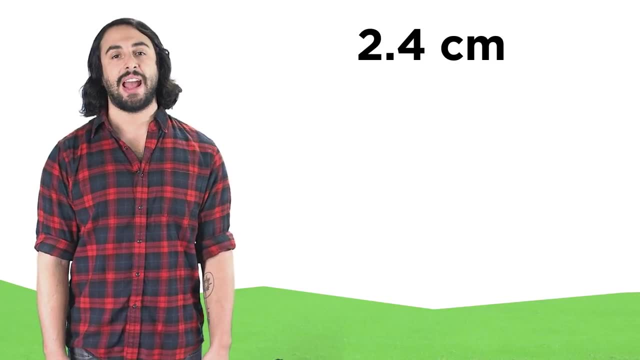 that is reported on the measurement. Let's look at the measuring instrument. The more digits there are in our measurement, the more precise it is. But no matter how precise our measurement, there will always be some uncertainty associated with it. If we measure something as being 2.4 centimeters, 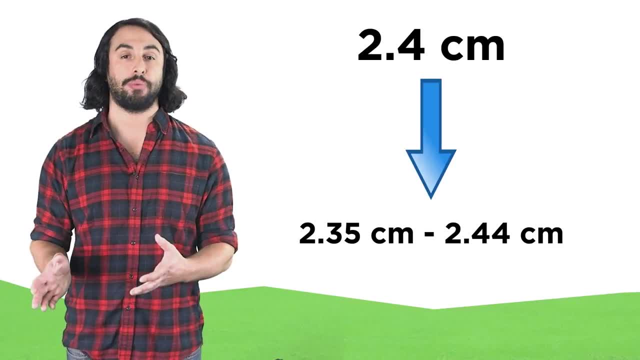 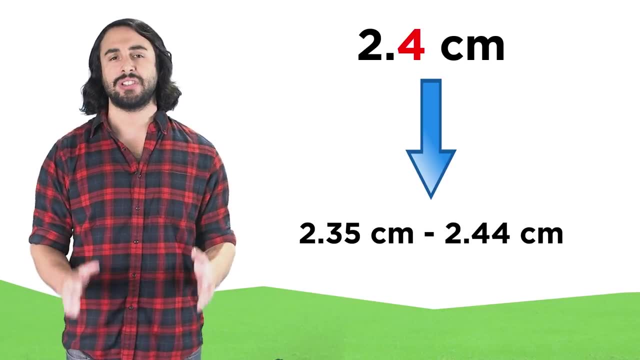 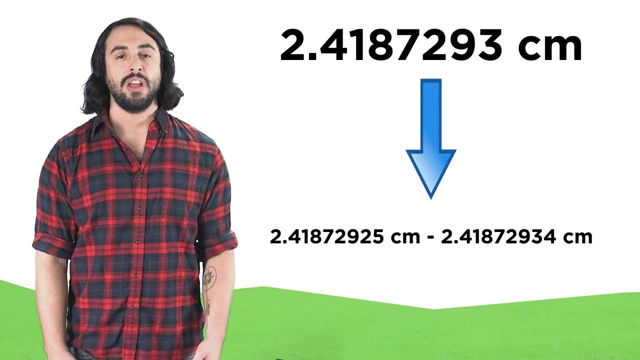 that means that it is really somewhere between 2.35 and 2.44, which will round to 2.4,. since the tenths place limits the precision. Even if it was 2.4187293 centimeters, there is still uncertainty associated with that. 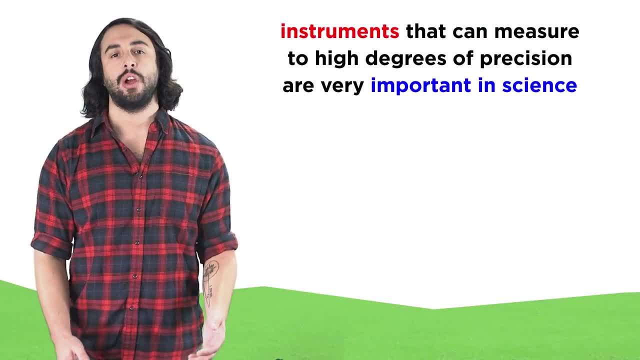 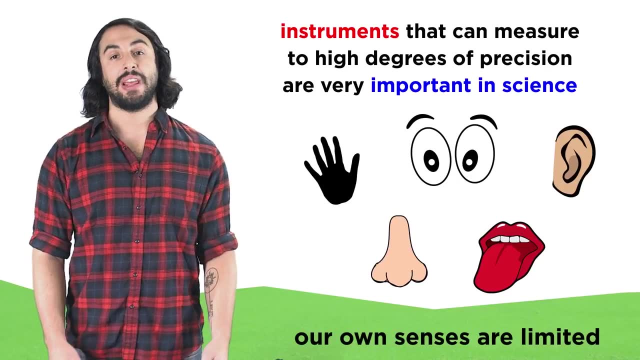 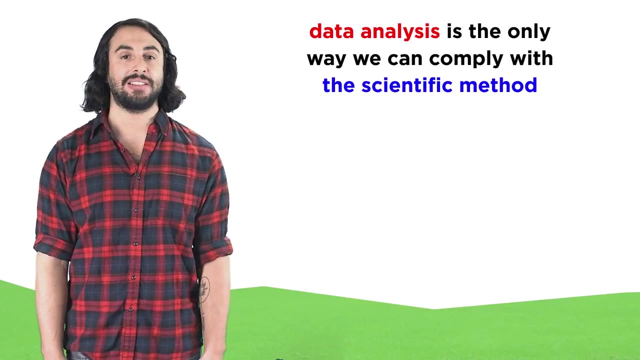 final digit. The precision associated with measurement is an important concept to understand, because we are limited by our five senses in the way that we interact with the world and therefore in how we do science, since analysis of the data we collect is the only way we can do science. 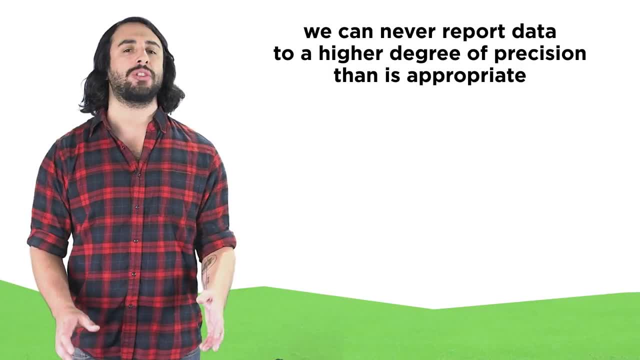 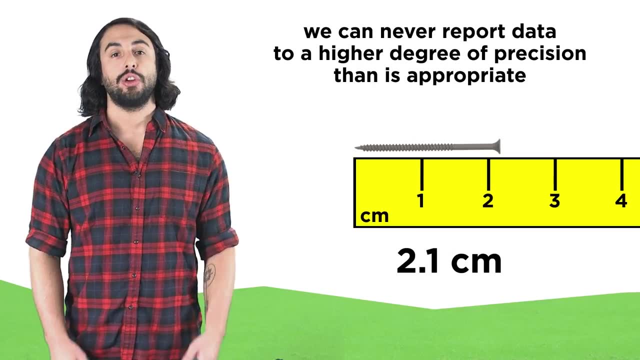 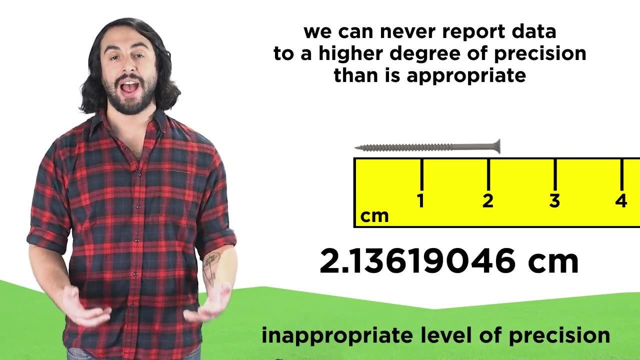 in the first place. We never want to report data to a higher degree of certainty than is appropriate, so that previous measurement to the tenths place can only be to the tenths place, as there is no way for our eyes to estimate with greater precision than that. 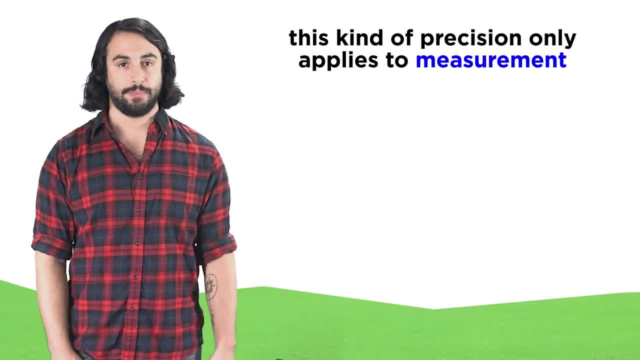 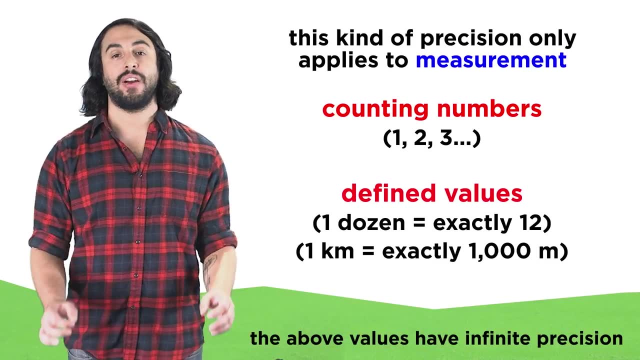 But this concept only applies to measurement. Counting numbers and defined values have infinite precision, like the way that there are exactly twelve in a dozen or exactly one thousand meters in a kilometer, with no uncertainty of any kind. The precision of measurements. 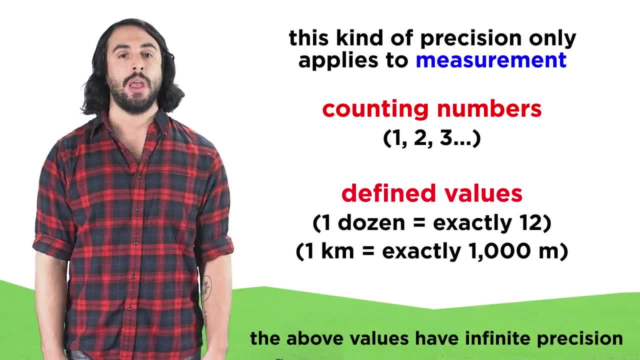 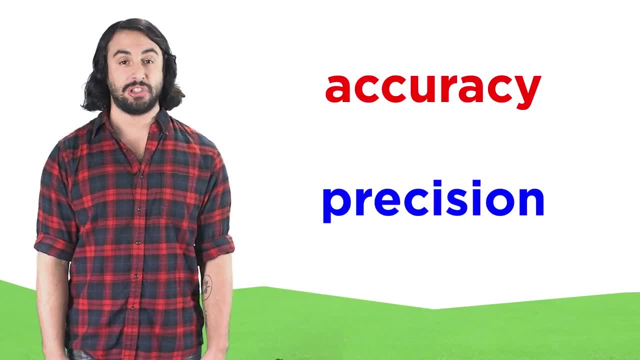 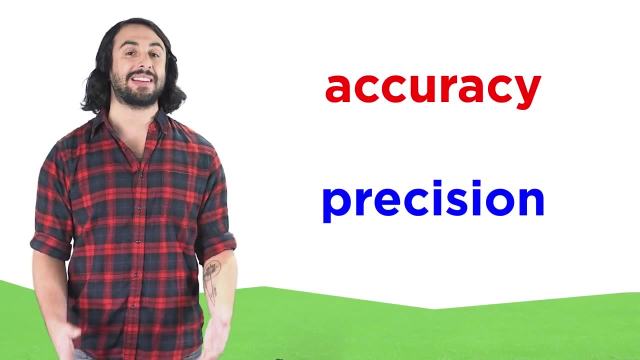 will affect the way we do calculations with our data, but these infinitely precise values will not. At any rate, accuracy and precision are important concepts to understand because, as we said, measurement is the way we collect data and the interpretation of this data is what science. 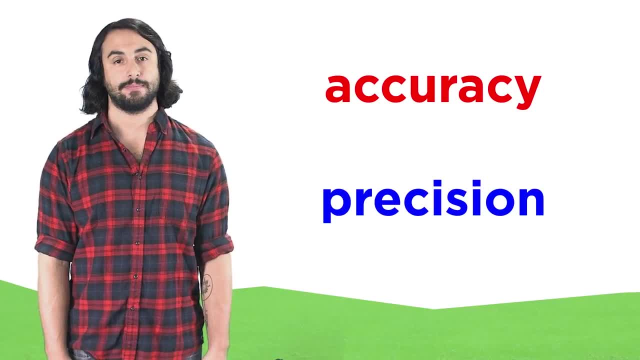 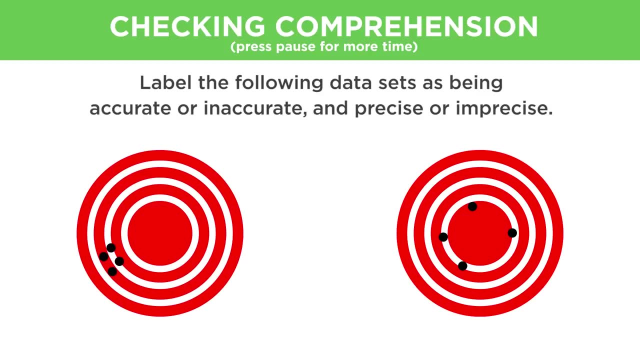 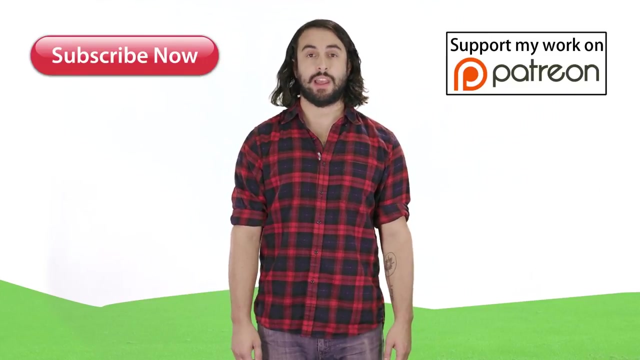 is really all about. Let's check comprehension. Thanks for watching, guys. Subscribe to my channel for more tutorials, support me on patreon so I can keep making content and, as always, feel free to email me. professordaveexplains.